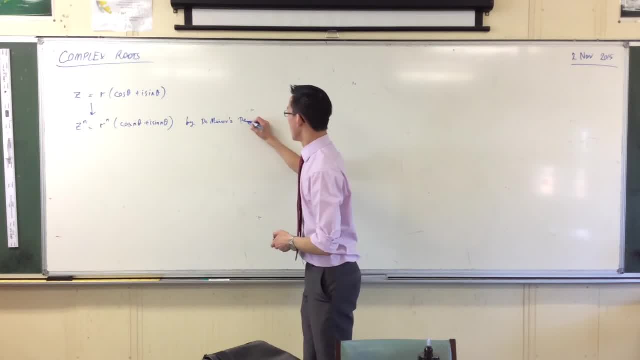 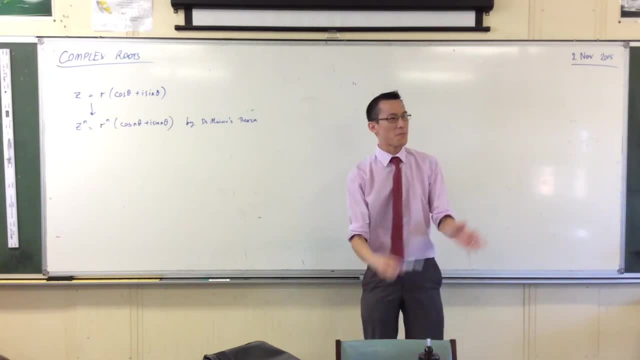 Now do we need to quote this- Which is why I'm writing it Now- when you can see we're going down in this direction? right, De Moivre's theorem gives you powers. gives you powers like raise to the power of 2,, 3,, 4,, 5, or even negative numbers. that's fine. 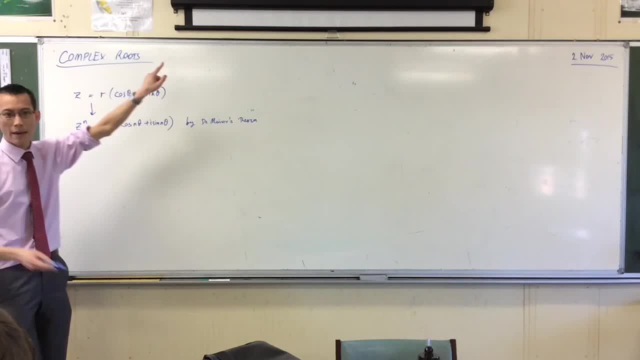 That's division, right, But complex roots roots. But complex roots is about going in the opposite direction. right, If I say square root or cube root or fourth root or whatever? right It's. instead of multiplying it's by having division, right. 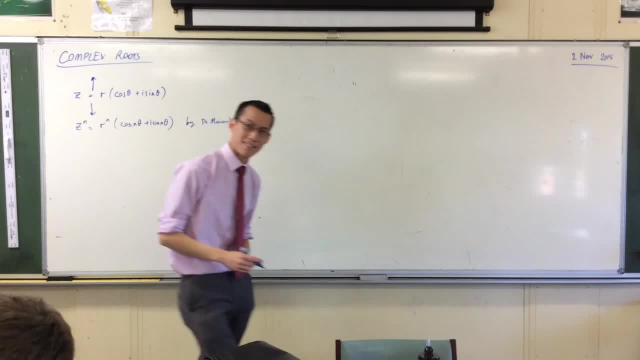 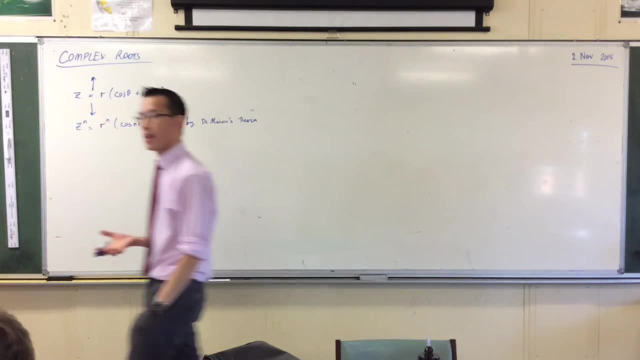 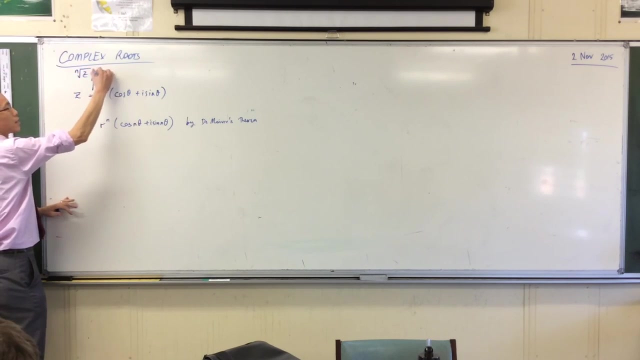 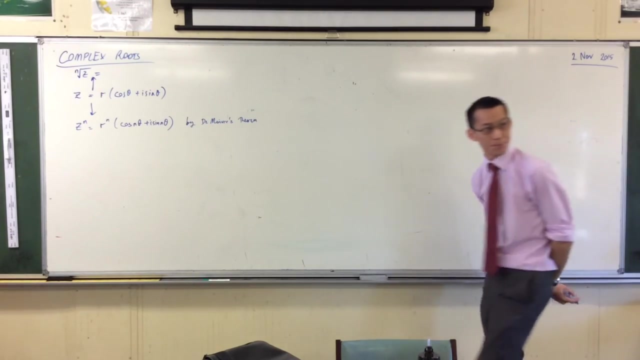 So if I go backwards, wow, why not? okay, Let's think about what we would guess to be the case if, instead of having the nth power of z, what if I had the nth root of z? What would you guess? De Moivre's theorem would kind of like generalize to, in this case, z to the power of 1 over n. 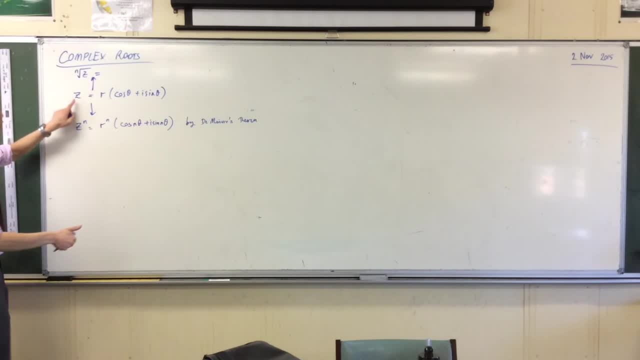 Okay, so that's just the index form, right? So here, because in index form this is z to the power of 1 over n, everywhere I have n in here I can replace it with 1 over n up here, right. 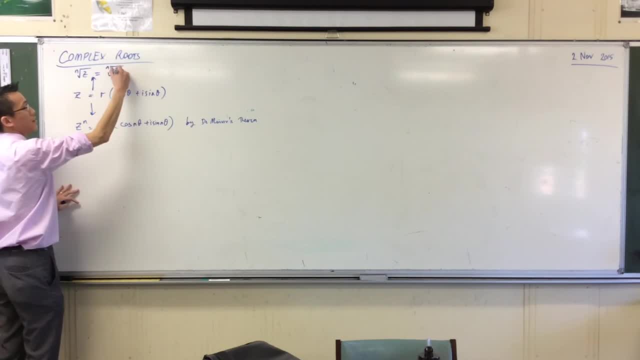 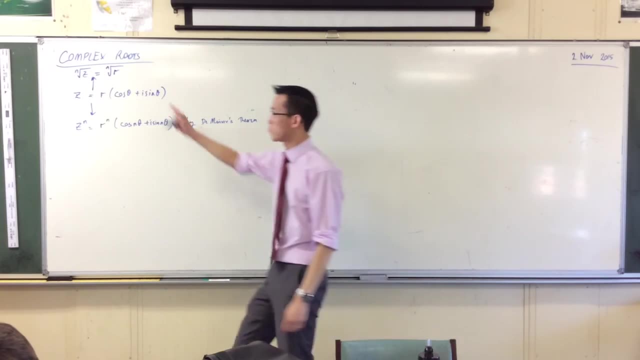 Is that okay? So I'm going to write that out just at the front, because r to the power of 1 over n is just the nth root of r. What about the arguments? What happens? We multiply mods. we should add arguments. so the opposite is division, right. 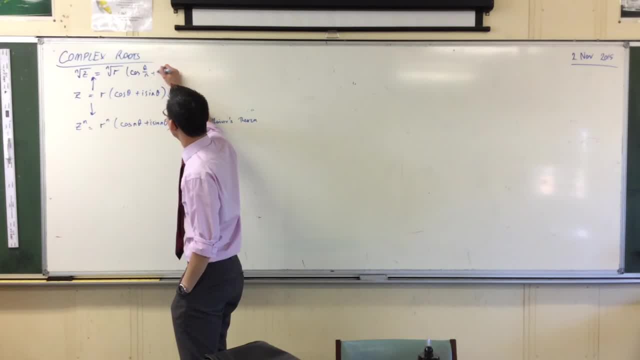 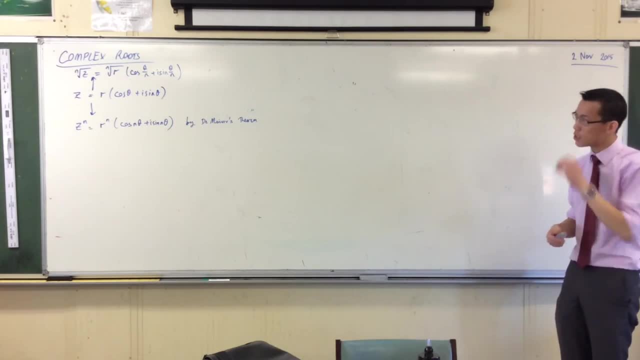 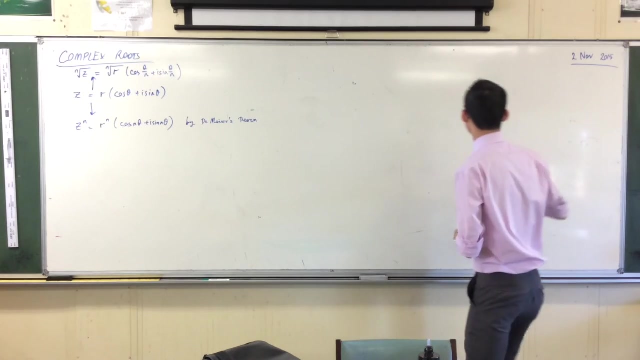 So I'm going to get this. Okay now, this is fine. This is true. Excuse me, There's nothing wrong on the board, It's just that it's not complete, right? So you know, when we talk about alright, what's the square root of 25, right? 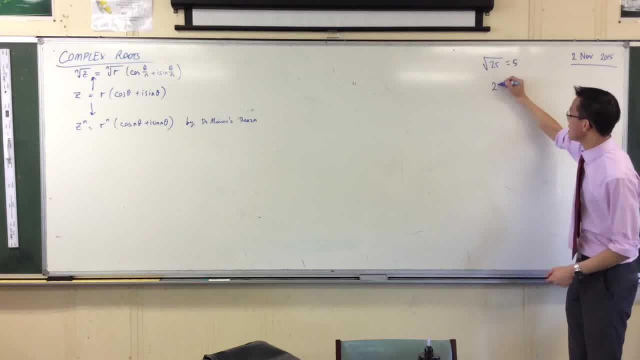 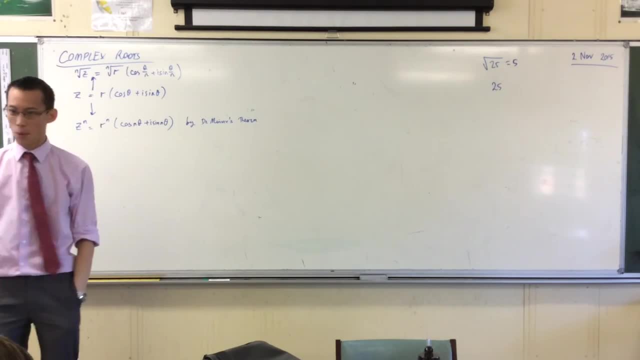 And the square root of 25 is 5. 5. 5. 25 has two numbers which are equally square roots. They're not the square root, but they're both numbers you can square. that will give you 25, right. 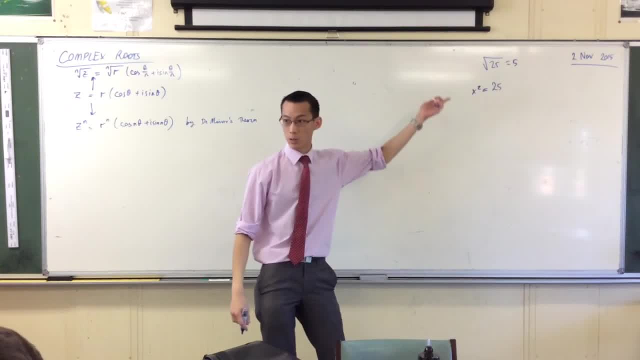 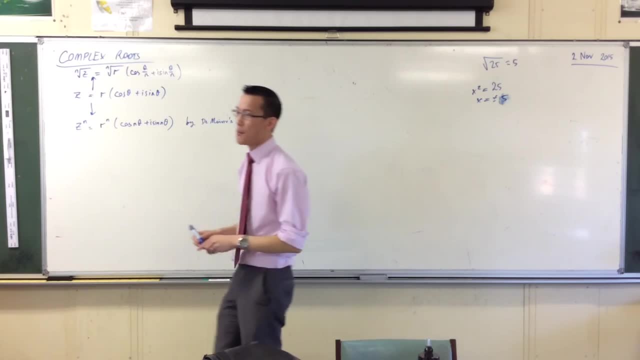 So, of course, the equation that would give you those two solutions is: x squared equals 25.. We know this is two answers, right, Whoops? So plus or minus 5 are both square roots of 25, right, But 5 is the square root. 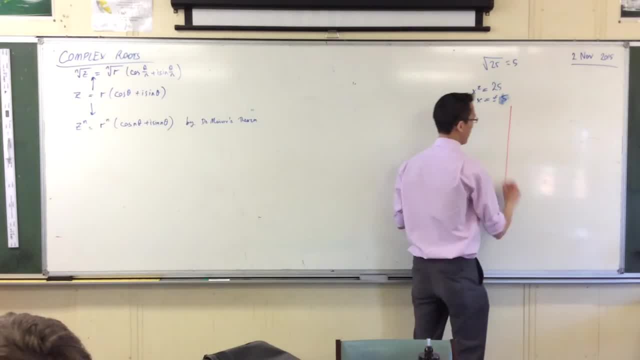 If you remember what we were talking about in the complex plane, we were talking about defining a number based on its modulus in its argument and we said, okay, if I have a number over here, okay, 1 plus i, or something like that. 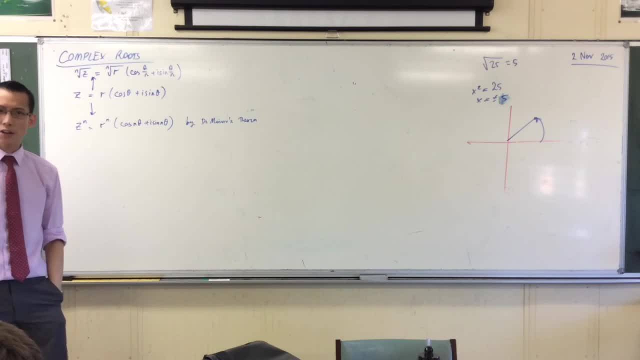 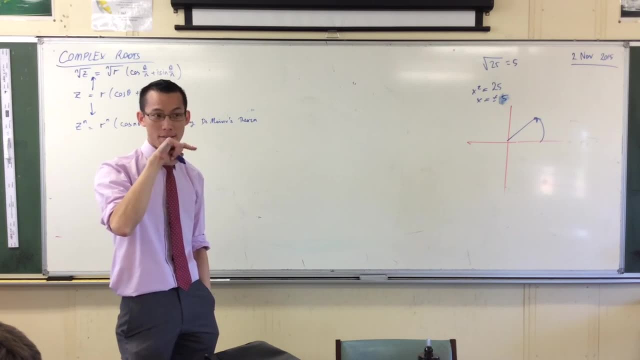 I could say its argument is pi over 4, but that's not the only argument I could use right Like: give me an example. What's another argument I could put on there? If I add multiples of, like, this is pi over 4,. 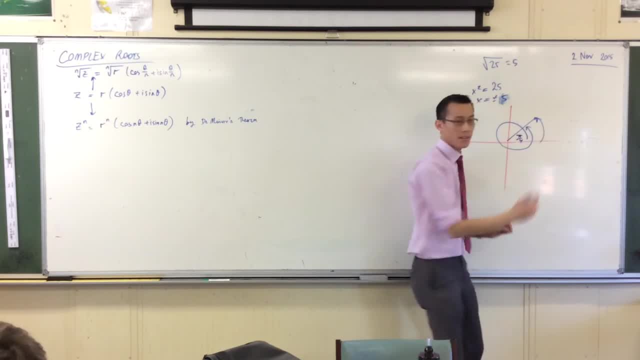 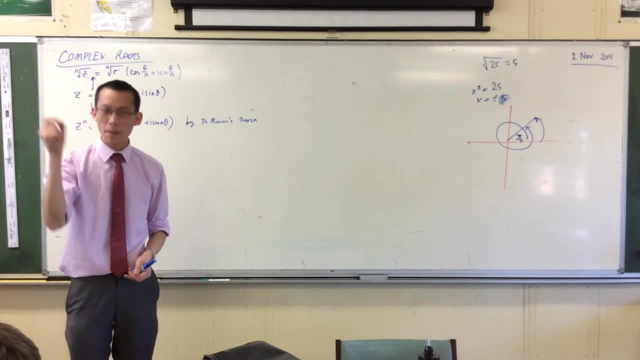 and if I go that angle and then add another 2pi, what's pi over 4 plus 2pi, 2 plus pi over 4.. 2pi is 8pi over 4, right, 2pi is 8pi over 4, so when you add it to that, pi over 4,. 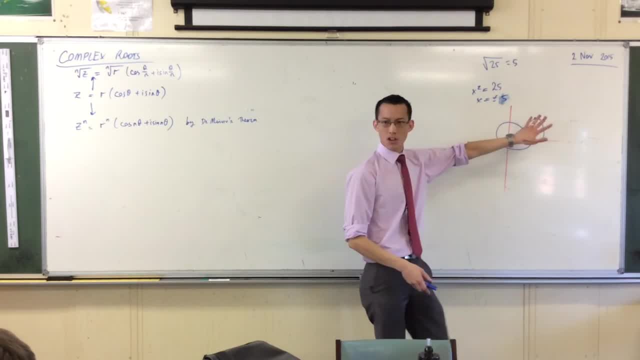 you'll get 9pi over 4, okay. So we have this non-unique representation. okay. So, just like I have a principal argument, I also have a principal square root. right, There's one which I consider like the main one, okay. 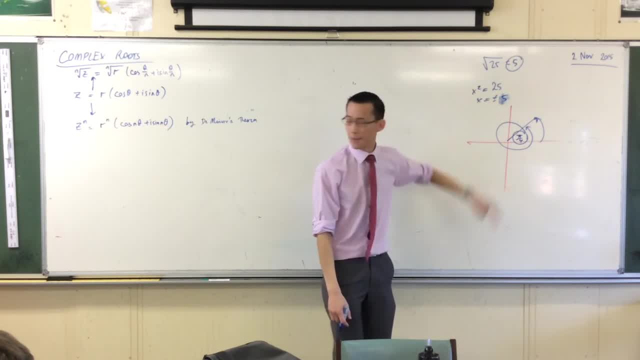 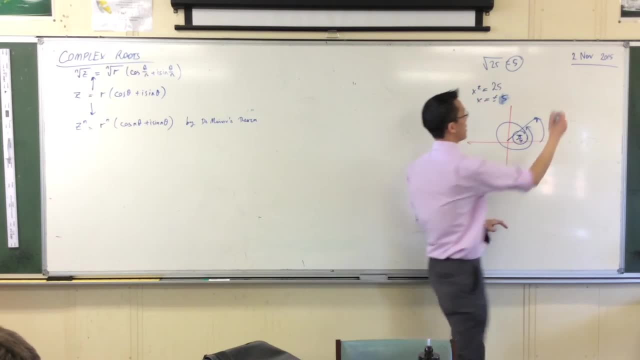 Even though there are others sort of hanging around on the side. okay, But when you look at complex numbers, things open up a lot more than this. right, A number has two square roots. What about if I asked you for how about this? 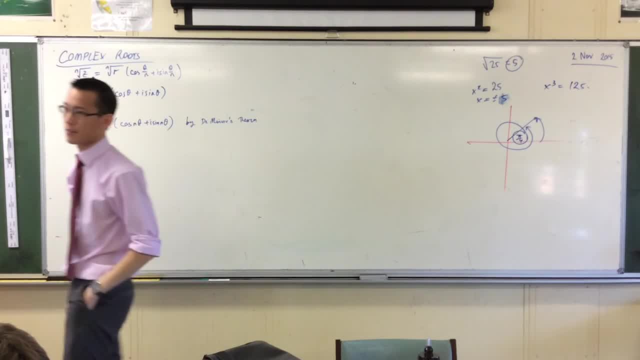 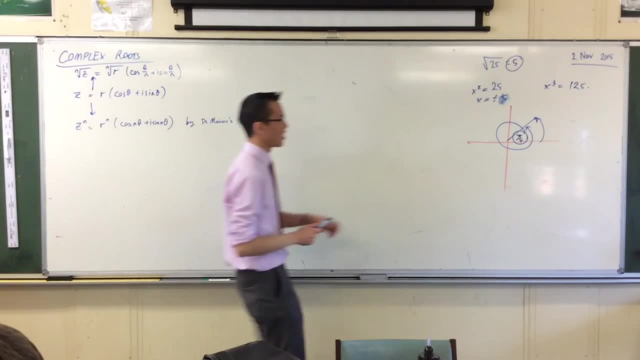 Okay, so this is just the same number, right? How many cube roots are there of 125? Three, There's one. One. How many There's four? Three, Now, interestingly, we would say: excuse me, in the real number world. 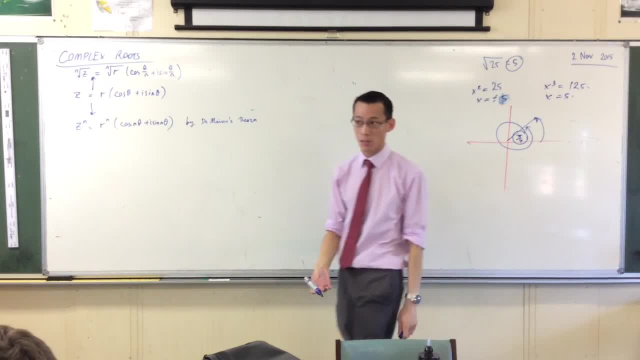 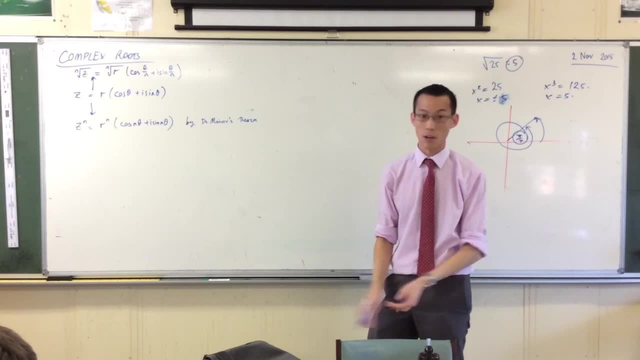 in the real number world I would say there's only one solution. right, There's only one solution. But we know in the complex world we find more okay. So to help unpack this, I'm going to show you an actual example. 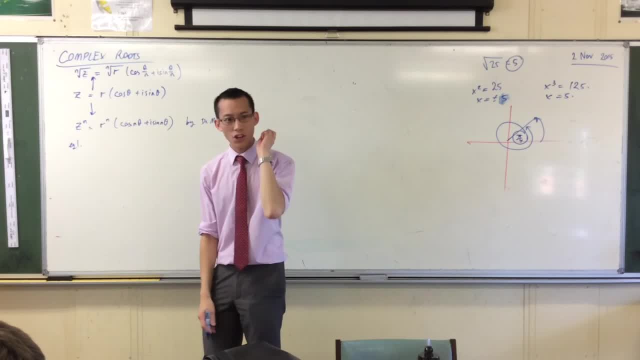 Let's find- here's an example. Let's find the cube root, because that's the one where that's the first time we're encountering, you know, this issue of how many roots are there. Let's find just the cube root of a nice simple, complex number. 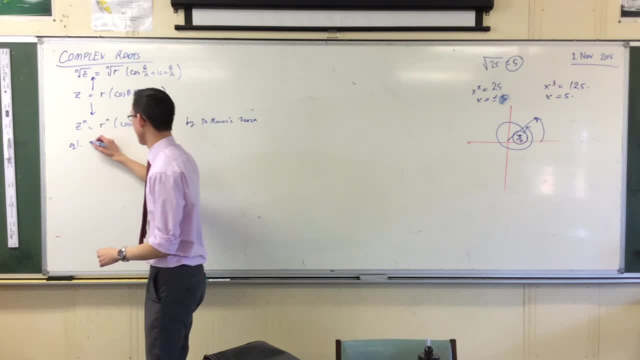 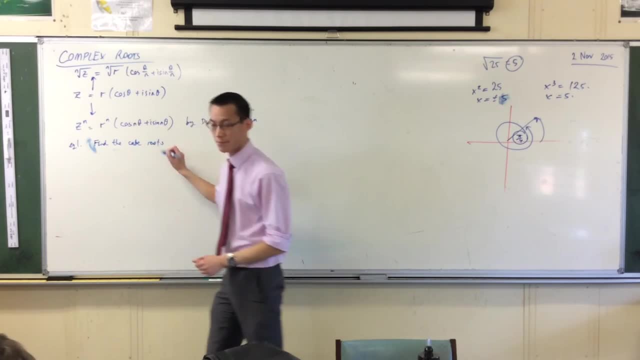 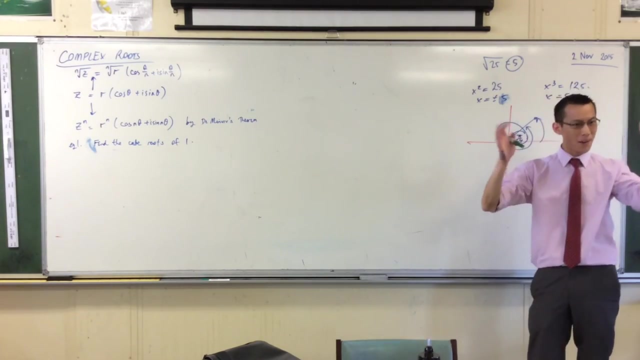 like say simple, complex number, like say one: okay, Find the cube roots and you'll notice I am saying plural of one. Okay, Now just a little side note, excuse me, the number one is an important number, right?